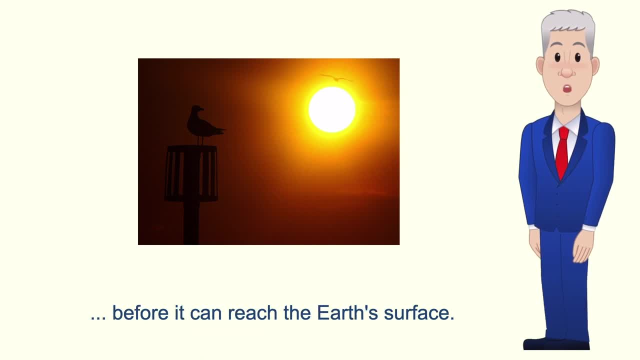 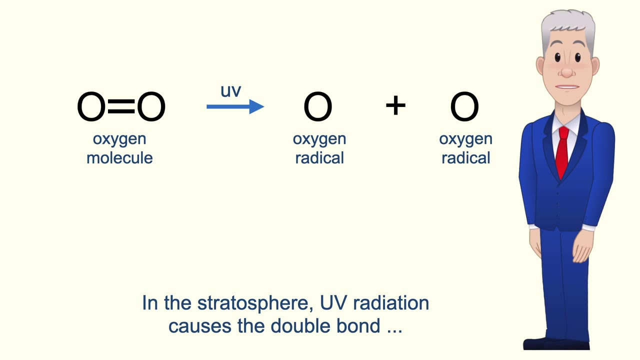 a great deal of the ultraviolet radiation from the sun before it can reach the earth's surface. so the ozone layer protects living organisms from excessive UV exposure. You need to be able to describe how the ozone layer does this. UV radiation causes the double bond in oxygen molecules to break, like this: 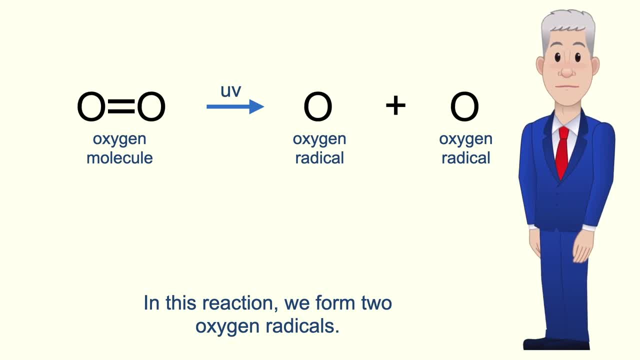 In this reaction we form two oxygen radicals, and remember that a radical is a species with an unpaired electron. You'll notice that I'm not showing the unpaired electron in the radicals, but you need to remember that they are still radicals. We can also show this reaction in a 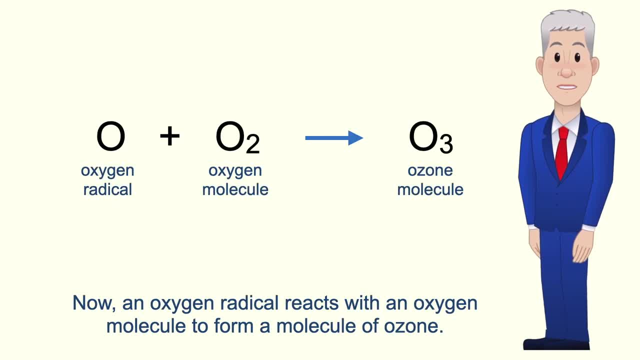 simpler form like this. Now, an oxygen radical reacts with an oxygen molecule to form a molecule of ozone. If this was the only reaction taking place, then ozone levels would continuously increase. However, an ozone molecule can absorb ultraviolet light. turning back to an oxygen radical and 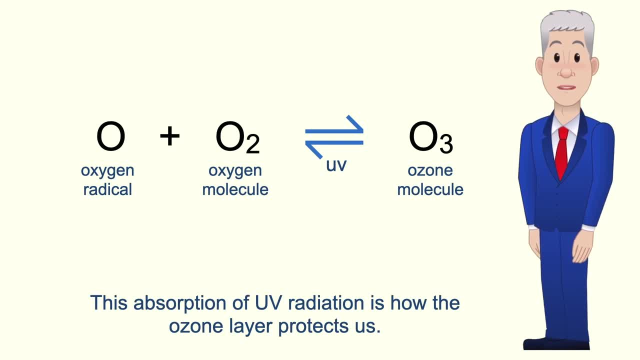 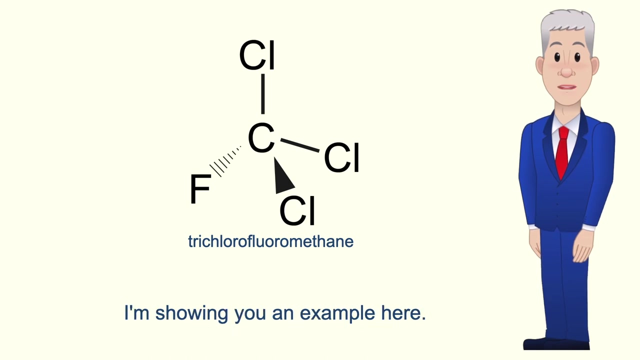 oxygen molecule. The absorption of UV radiation protects the ozone layer Because ozone is formed and broken down at the same rate. the amount of ozone in the ozone layer should remain constant. However, certain chemicals can cause ozone in the ozone to be broken down. These chemicals are called chlorofluorocarbons or CFCs, and I'm showing 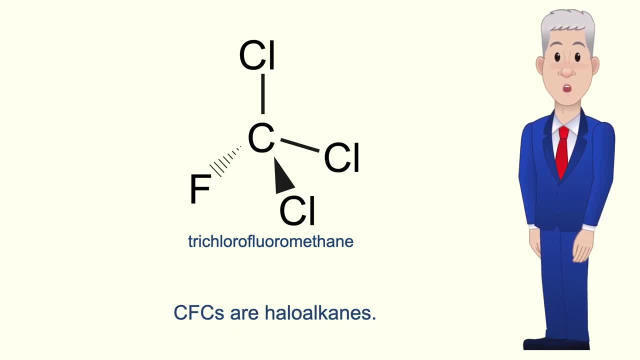 an example here: CFCs are haloalkanes. Now, CFCs are very stable molecules and that's because of the high bond enthalpy of the carbon-to-halogen bonds. CFCs are also relatively non-toxic. 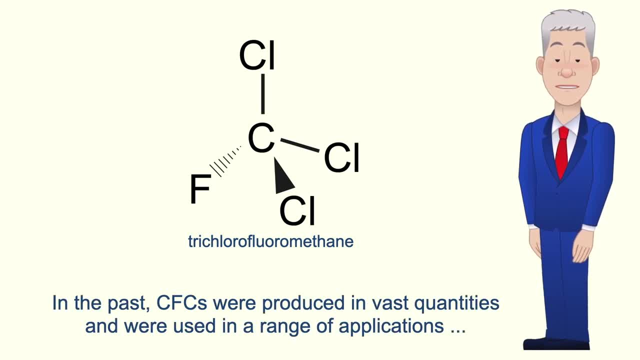 In the past, CFCs were produced in vast quantities and were used in a range of applications, for example in fridges and freezers. However, scientists later discovered that CFCs could cause the destruction of the ozone layer. CFCs make their way up to the stratosphere. 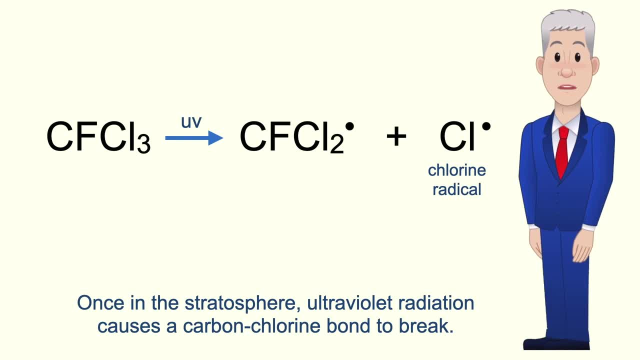 Once in the stratosphere, ultraviolet radiation causes a carbon-to-chlorine bond to break. Scientists call this process photodissociation. This is homolytic fission and produces a chlorine radical which is highly reactive. The next stage involves two steps.